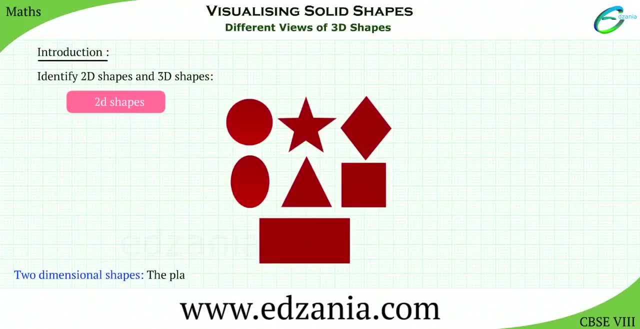 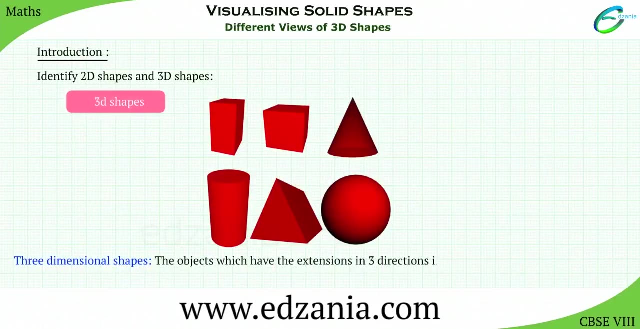 Two-dimensional Shapes: The plane shapes have two measurements, like length and breadth. They are called 2D shapes. Three-dimensional shapes: the objects which have the extensions in three directions, that is, length, breadth and height, are called three-dimensional shapes. Three-dimensional objects have thickness. 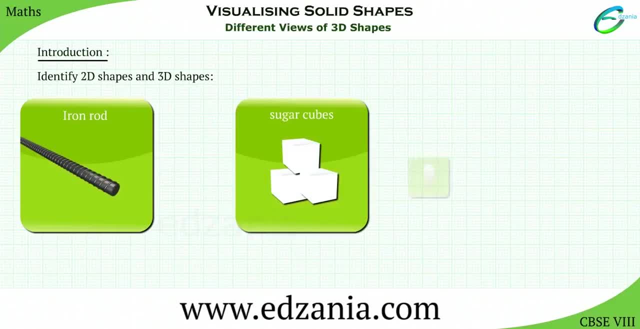 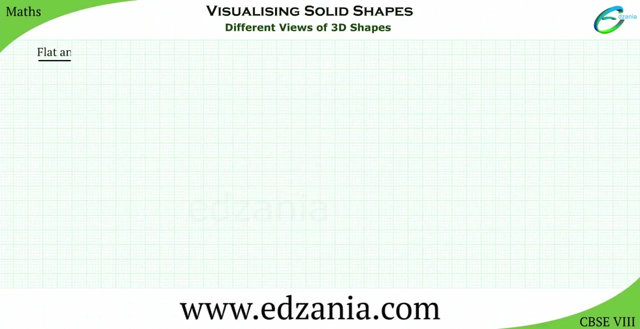 Iron rod, sugar cubes, cone. these are all solids because they have volume, that is, they occupy space. The solids are also called three-dimensional objects. Three-dimensional objects have different plane surfaces. Let us observe the plane surfaces of objects. While touching the surface of a book, we feel flat surface. 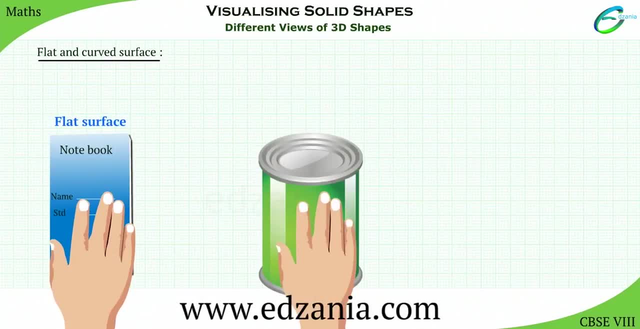 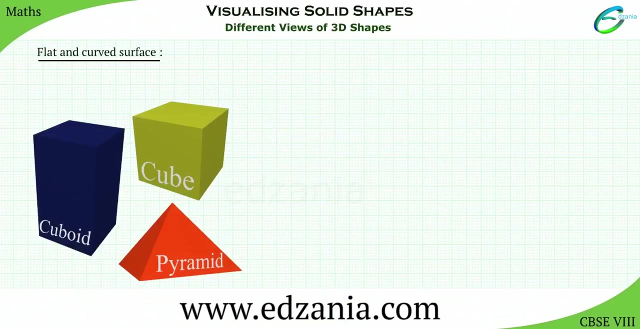 Similarly, while touching the surface of a cylindrical tin, we feel different surface. Can you tell me what is that surface of the tin? Curved surface. Look here, there are some 3D shapes which have flat surface, Some of the 3D shapes which have curved surface. 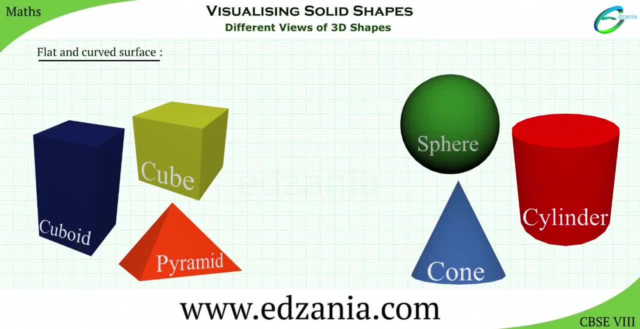 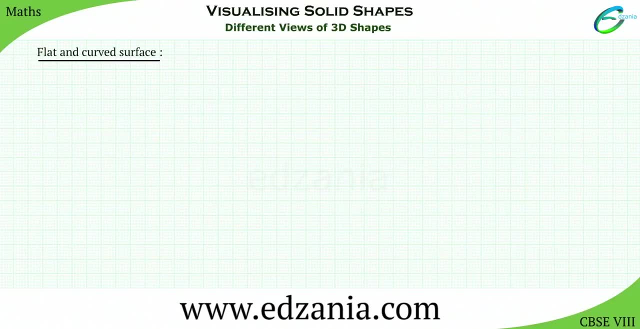 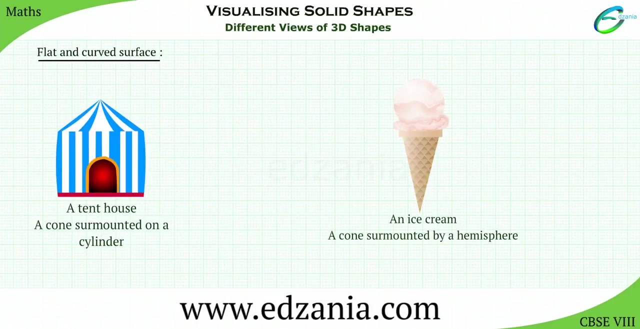 Some 3D shapes have flat surfaces. Some 3D shapes have curved surfaces. Let us look into some of the objects which are surmounted by another 3D object: A tent house, a cone surmounted on a cylinder, An ice cream. a cone surmounted by a hemisphere. 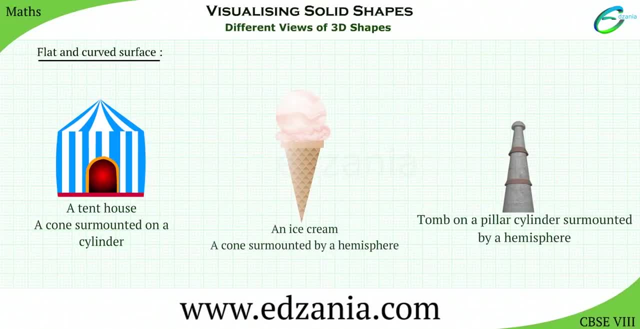 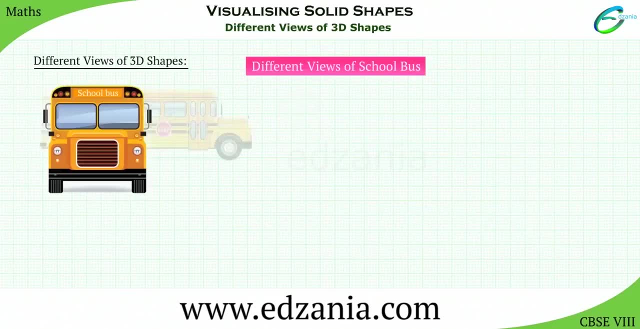 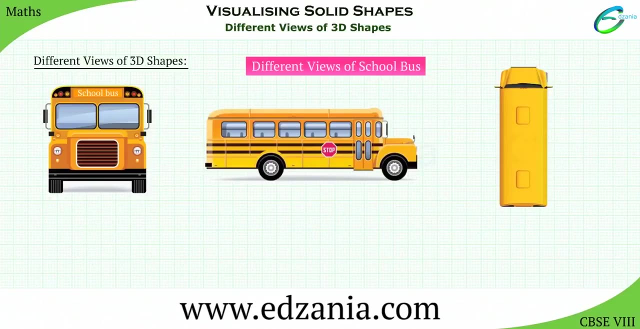 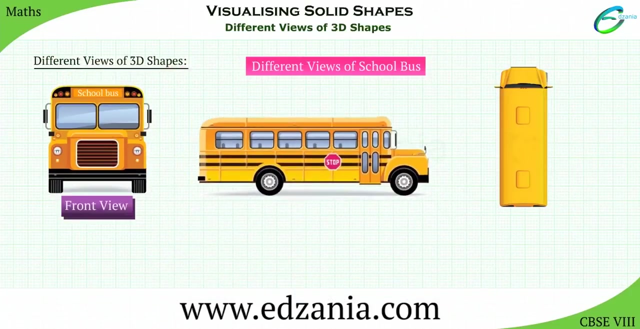 Tomb on a pillar cylinder surmounted by a hemisphere. You have seen some of the 3D objects and solids. 3D objects view differently in different views. Look at the school bus: The view from the front, the view from the side and the view from the top. 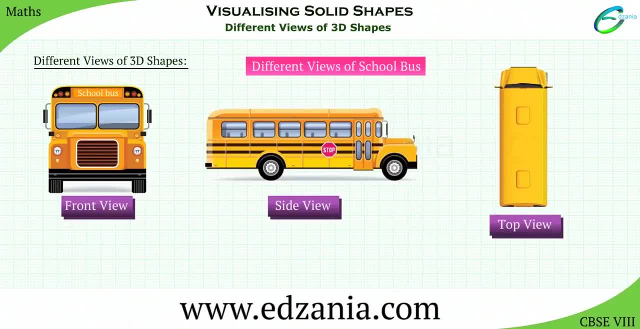 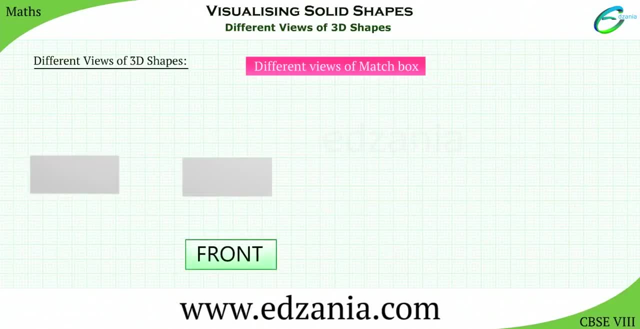 These are the different views of the bus. Observe the different views of the matchbox: Front view of the matchbox, Side view of the matchbox And the top view of the matchbox. Here it is a solid made of 3 cubes.